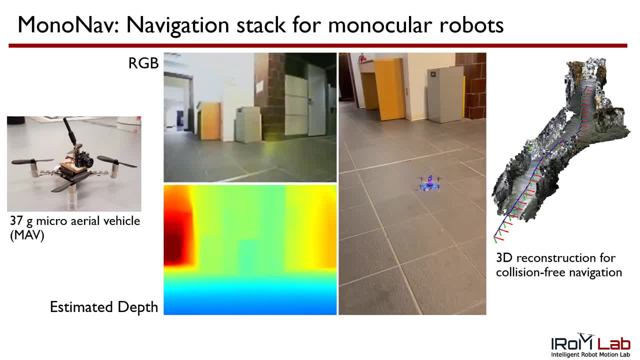 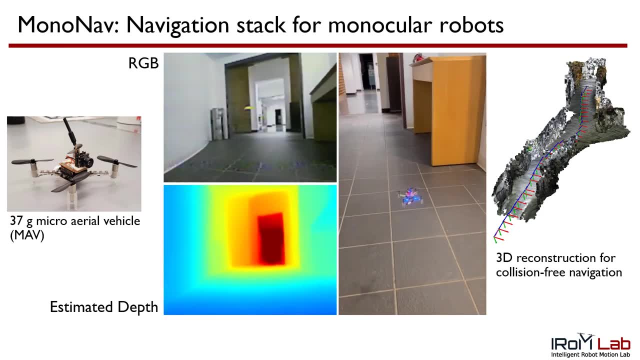 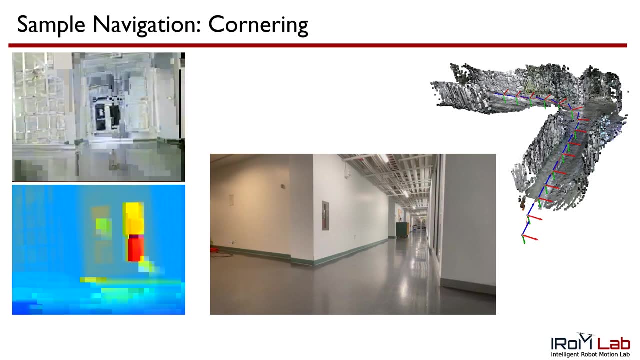 state-of-the-art metric depth estimation networks, off-the-shelf fusion algorithms and conventional planning techniques to enable tiny monocular robots to navigate fast and constrained indoor environments. Here we see MonoNav navigating a hallway with a curved wall on the left and furniture ahead. In another example, MonoNav successfully. 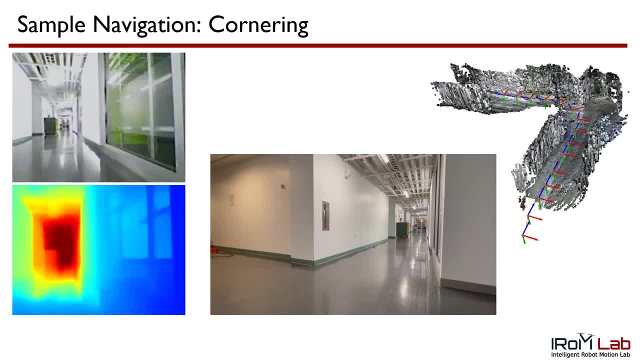 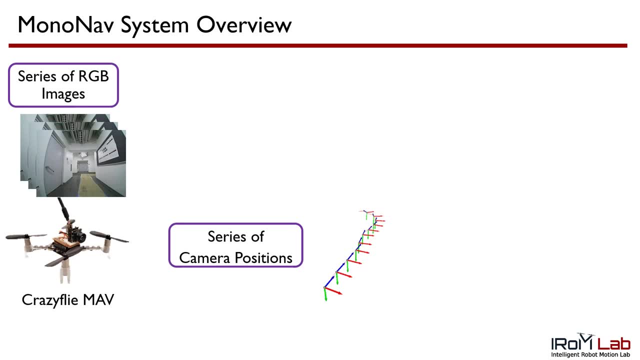 navigates a corner at 0.5 meters per second. In real-time, MonoNav generates a 3D reconstruction which it uses for planning. MonoNav starts with a series of monocular images, which are monocular images, and camera poses, which are readily available to the Mav. We use Zoidep, a pre-trained 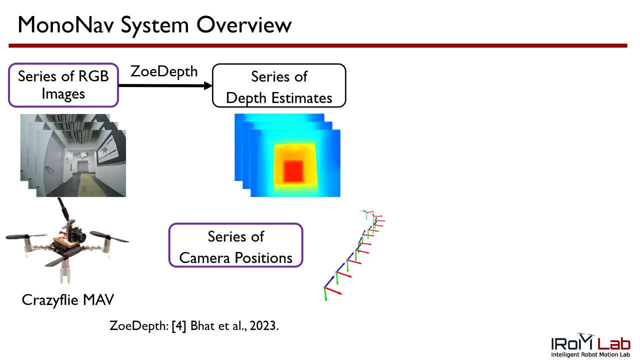 network to perform per-frame metric depth estimation. Next, we integrate the depth estimates and poses into a 3D reconstruction using Open3D For planning. we consider a library of motion primitives generated offline Using the 3D reconstruction. we select a collision-free. 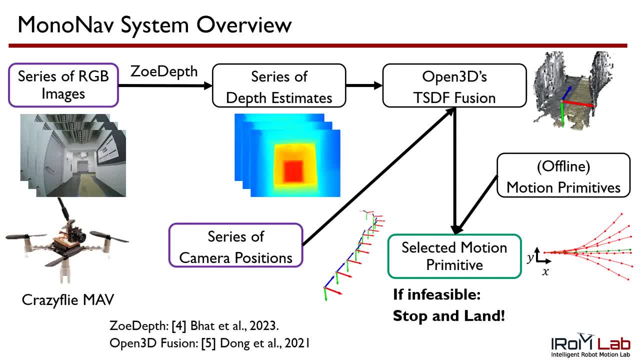 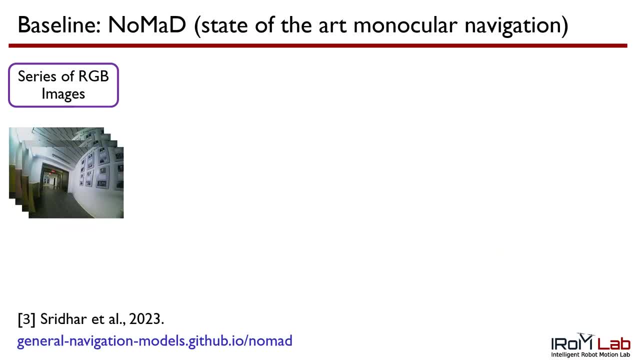 motion primitive. If the motion primitive selection problem is infeasible- in other words no primitive is collision-free- then MonoNav executes a safety maneuver. We compare MonoNav to Nomad, the state-of-the-art in monocular navigation. Nomad runs a series. 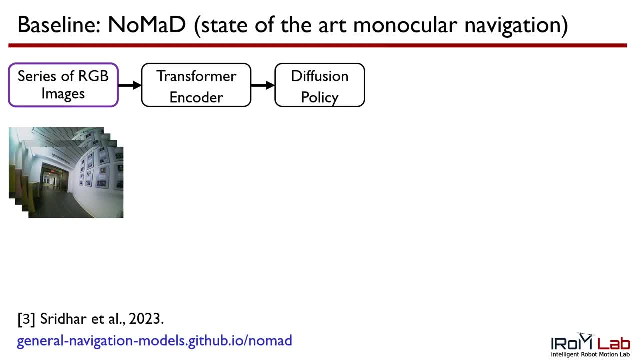 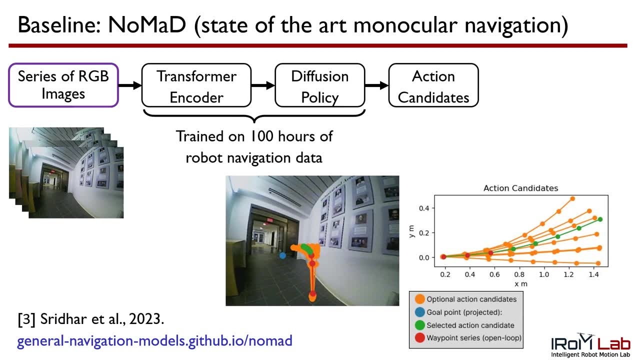 of monocular frames into a transformer encoder and a diffusion policy trained on 100 hours of robot navigation data. The diffusion policy directly outputs action candidates as position trajectories. Since all candidates should be collision-free, we choose the action that makes the most progress towards the goal and execute the first three waypoints before replanning. 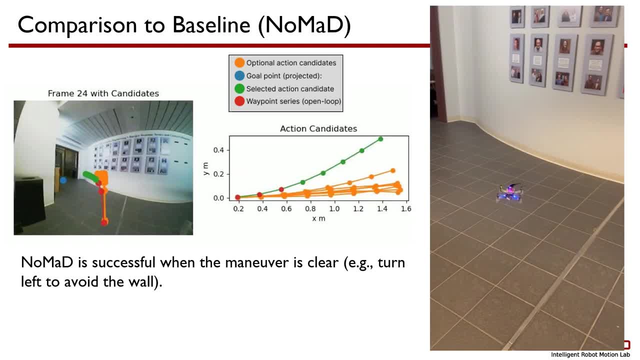 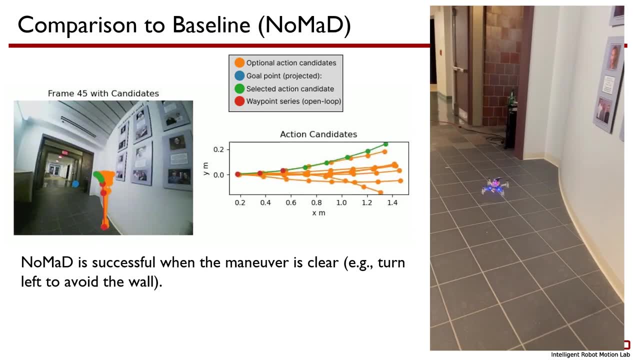 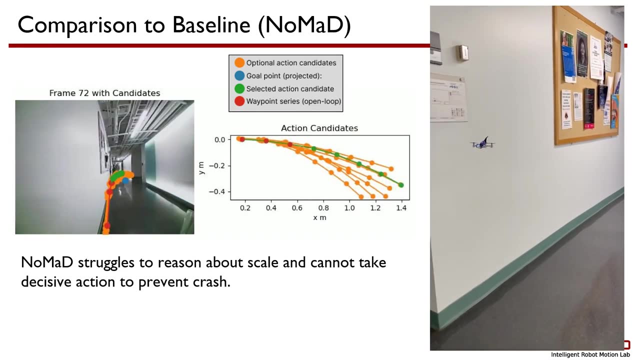 In some cases the action candidates are very diverse and occasionally, inexplicably, suggest to turn into the wall. In another example, down a straight hallway, Nomad struggles to reason about scale and cannot take decisive action to prevent a crash. In this case, all 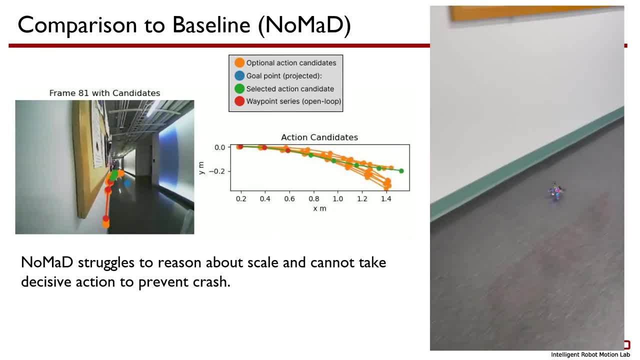 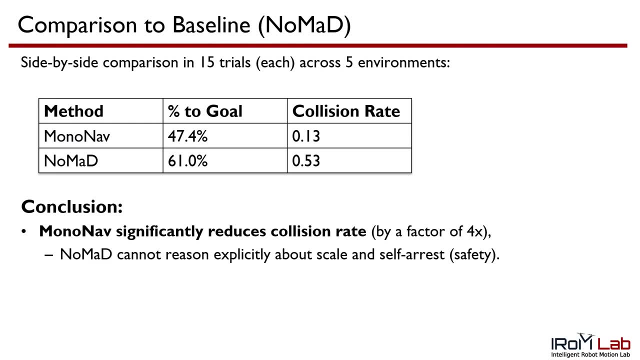 of the action candidates are very straight, which is not sufficiently evasive. We compare MonoNav and Nomad side-by-side in 15 trials and find that MonoNav significantly reduces. However, this improvement in safety comes at the cost of a 22% reduction in goal completion. 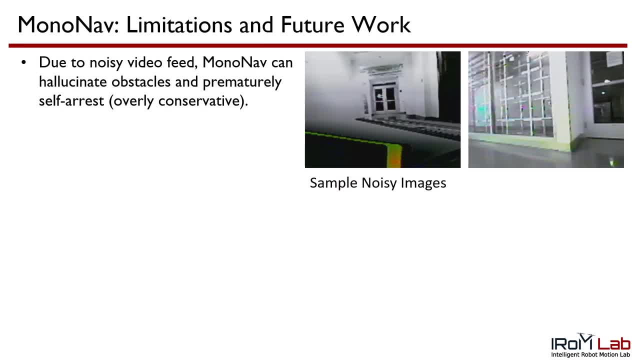 There are several limitations to MonoNav that merit future work. Due to noise in the image feed, MonoNav can hallucinate obstacles and prematurely self-arrest, which is overly conservative. In addition, the reconstruction quality is sensitive to errors in state estimation.